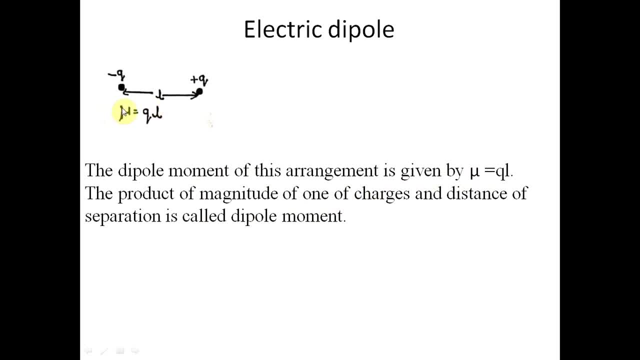 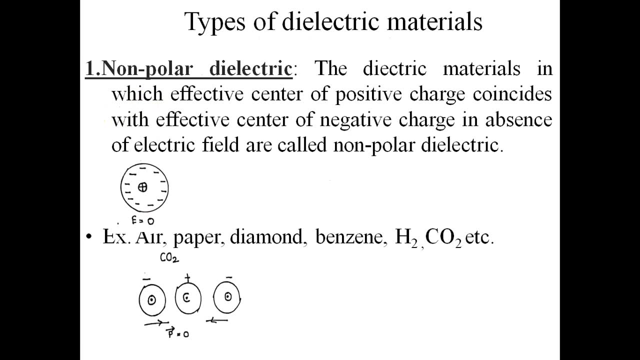 The difference in pellet charge to diametral charge, turn off charges and distance of separation is called as Dipole moment. There are two types of dipoles moment. The nonpolar dielectrics have the symmetrical inch shape. Now let us see the nonpolar dielectrics. 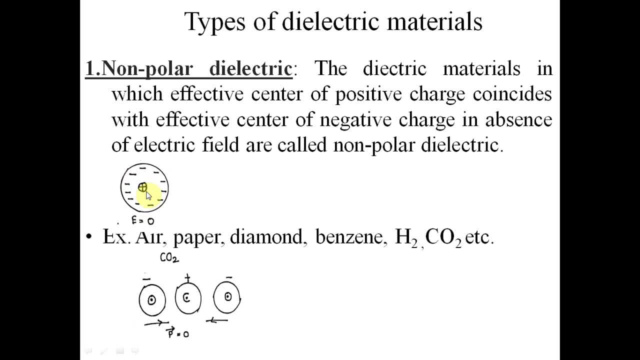 The Non-polar dielectrics have the symmetrical inch shape in which the effective center of this positive charge with a negative charge are coincide. in the absence of electric field is called as a non-polar dielectric. examples are air, paper, diamond, benzene, h2o, co2, etc. let us take one example, that one is the co2, o is oxygen. this 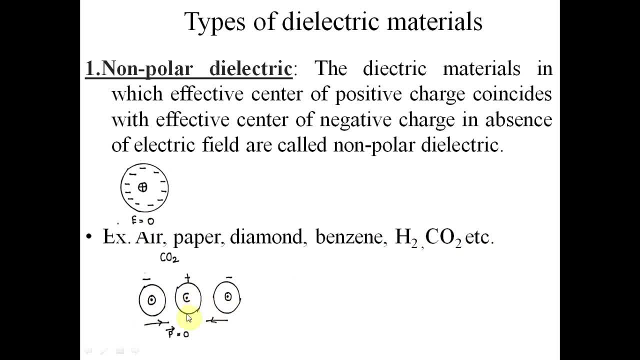 one: o is oxygen, c stands for the carbon, o is negative, o is negative. this c is the positive c. the center of mass of this o is here and this center of mass of is here and the center of mass of this c is here, then the both of this center of mass of this o is here means the center of mass. 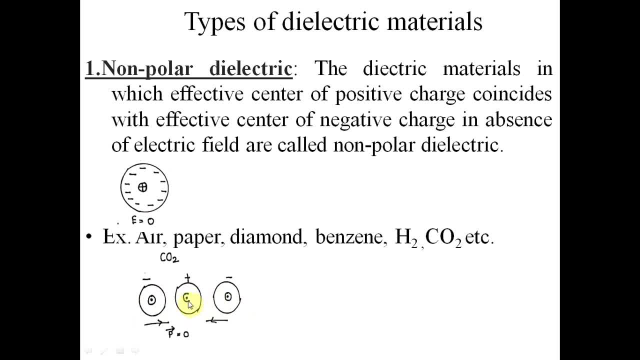 of this, c at the positive and center of mass of this negative, is coincided. coincide at this place means the both the dipoles are both the dipoles are opposite and cancels, hence the dipole moments p equal to zero. both they are coincided at one place. hence it is the non-polar dielectrics. now let us see. 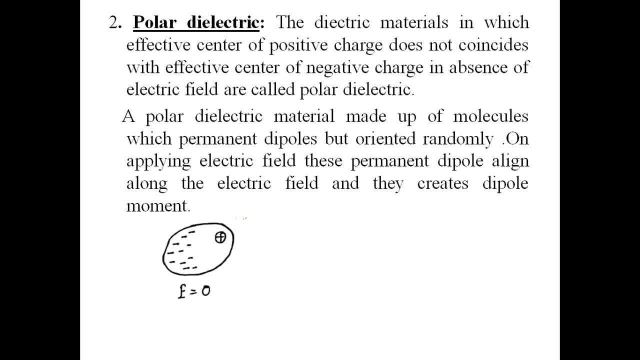 the polar dielectrics. polar dielectrics are symmetrical in shape. this dielectric, in which, if a two center of this positive does not coincide with this negative, charges in the absence of electric field, is called as the polar dielectrics, a polar dielectric materials made up of a molecule. 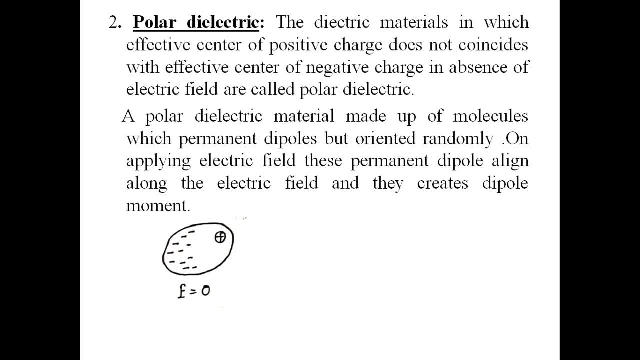 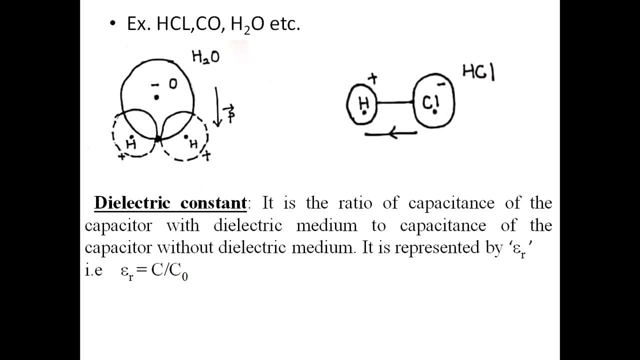 which, having there are the permanent dipoles, but oriented randomly on applying the electric field. these dipoles align with their electric field and they creates their dipole moments. now let us see example of this. one is take here h2o. you can see from this figure that the center of mass of this 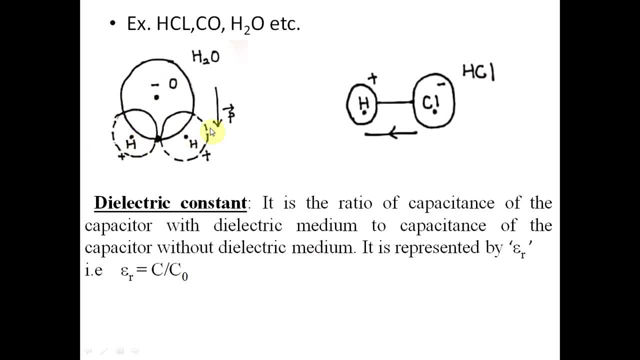 positive is here. the center of mass of this one is the positive is here. then o is stand for the oxygen, h is for the hydrogen. now both of this center of mass is here. okay, now that one, this center of mass of negative, is here, then there is a separation bit created between this negative to positive. there is a gap, is. 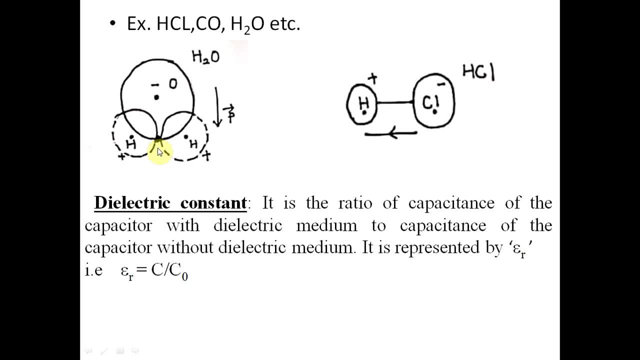 formation between this negative to positive, and so the dipole moments, it is from the negative to positive. similarly, here is a separation between this one is hcl also. so there is the negative and positive are not coincide in this non-polar polar dielectrics molecules. next one is the dielectric constant. dielectric constant, it is the ratio of capacitance. 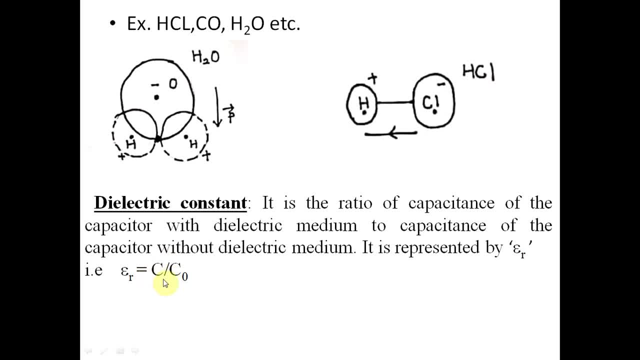 of the capacitor with the dielectric medium with the capacitance of the capacitor without the dielectric material, is called as the dielectric constant. it is represented as epsilon r, where c is this. c is the capacitance of the capacitor with dielectric cap. c 0 is the capacitor of the 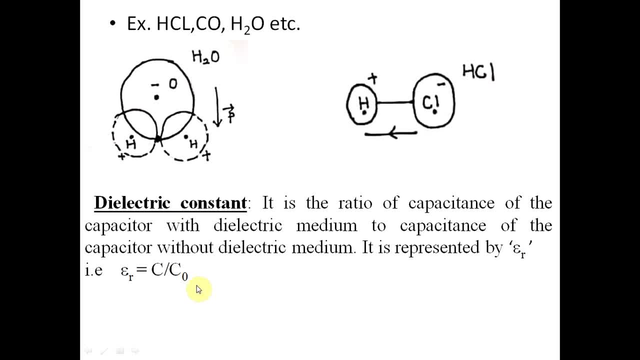 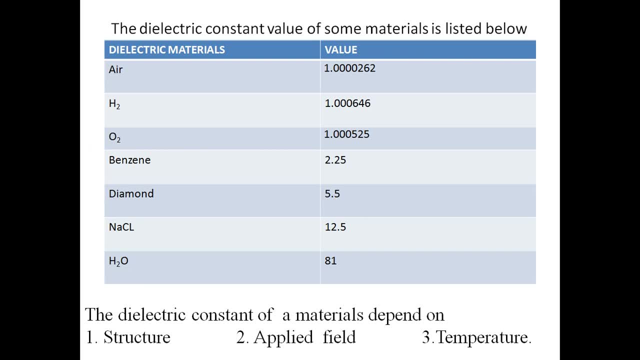 capacitance without dielectric and epsilon r is called as the relative permittivity and there are some dielectric constant values of some material are listed below. see there are. the list are for the dielectric materials and give their respective values. now see the for a benzene. it is the value it. 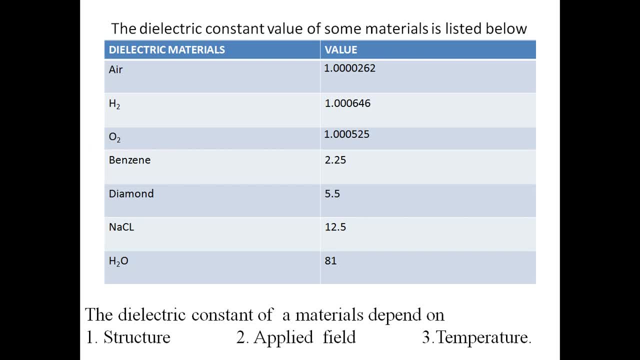 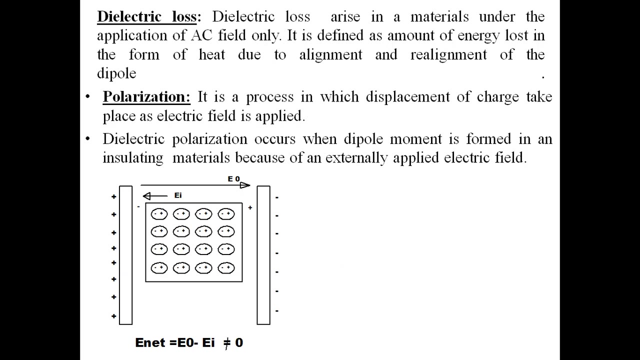 5. for the diamond it is 5.5. ncl is a 12.5, s2 is a 81. these dielectric constants are material. depends upon the structure, applied field and the temperature. next one is dielectric loss: the dielectric loss: it is defined as the amount of energy lost in the form of a heat due to the 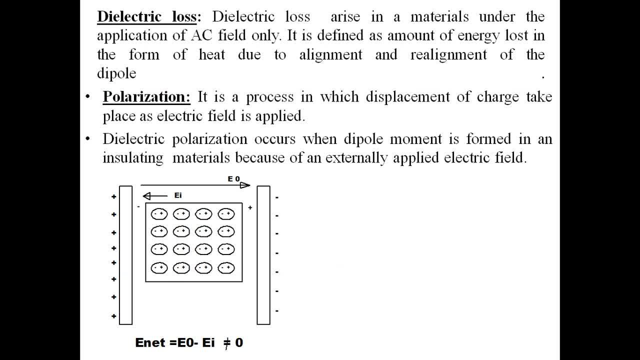 alignment, on the realignment of these dipoles, and this loss arise in the material under the application of their ac field. only now come to the next point is polarization. now see in this diagram, we take the two plates: okay, one with the positive and other one with. 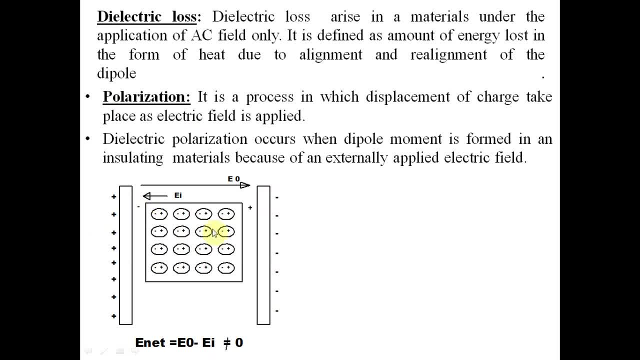 in negative charge now in between these two plates. place the dielectric between these two plates. now the dielectric is influenced to the electric field. okay, now the negative charge is a placed at one side, negative charge is placed at one side and positive charge it is a placed at other side. on this condition, positive to negative- there is. 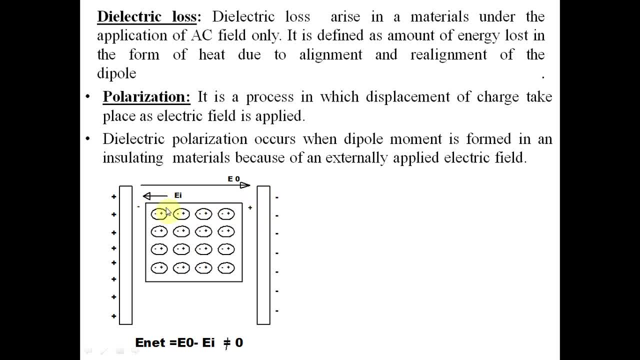 induced electric field is produced, positive to negative induced electric field, ei, is produced. now we can find the e net equal to e0 minus ei. both are opposite in direction and they subtract. but in dielectric produced induced electric field is weak. induced electric field cannot cancel to external electric field. it cannot cancel to 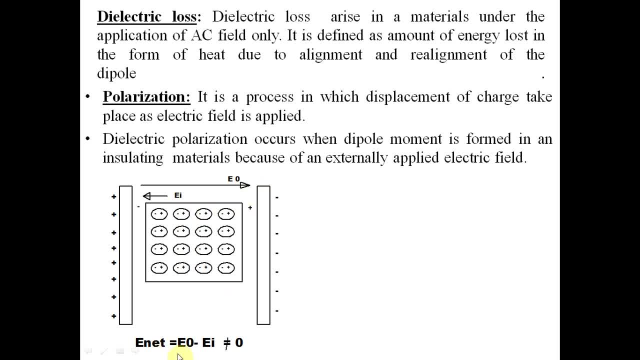 external electric field. so the value is e net equal to e0 minus ei. epsilon- not sorry, is not yellow. due to this e net some energy is stored in present inside this plate. that energy is stored it in capacitor, in dielectric. no free electrons. they are very tightly bounded. the atoms are little. 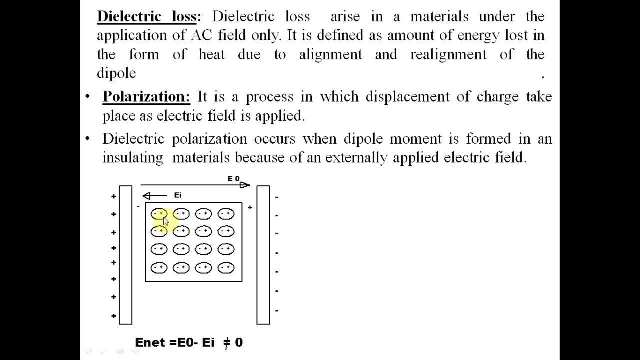 bit displaced. these atoms are a little bit displaced or just like a. it is called as alignment inside the item negative charge goes to the positive charge, charge okay. and this positive charge is goes, charge goes away. similarly, the next atom, likewise, like all the atoms, are little bit displaced or just like a stretch: negative at one side and the. 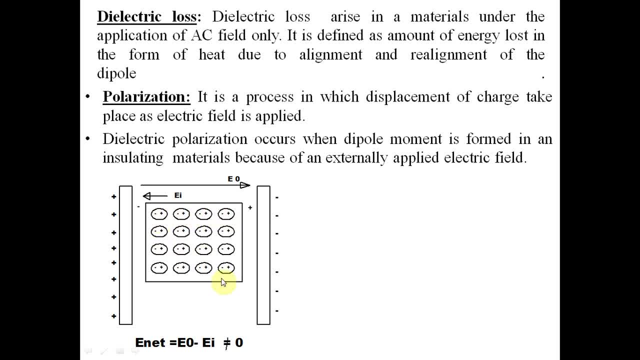 positive at other side and the alignment is takes place. that one is. the new word is coming that is called as the polarization. polarization, it is the process in which displacement of the charges takes place as the electric field is applied. the dielectric polarization occurs when the dipole 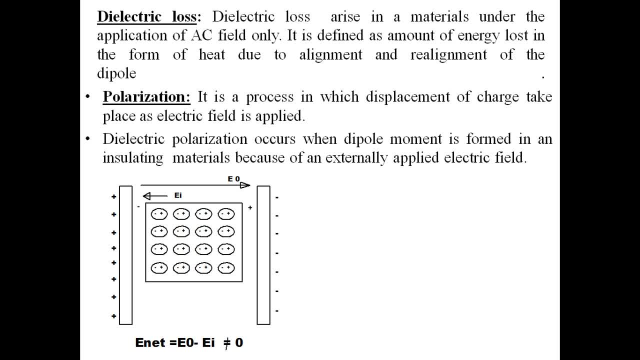 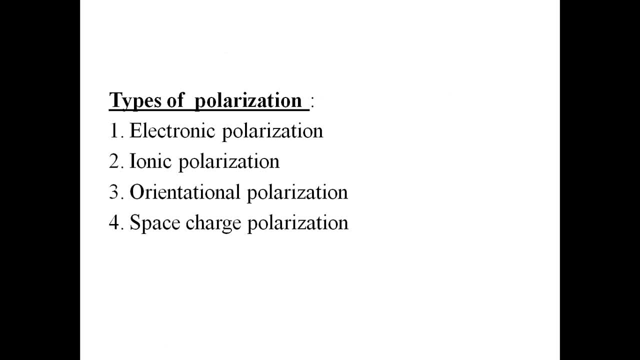 moment is formed in an insulating material because of an external applied electric field. so there are the four types of dielectric polarization. mechanisms are there. so first one is electronic polarization, ionic polarization and then the dielectric polarization. so these are the four types of dielectric polarization. 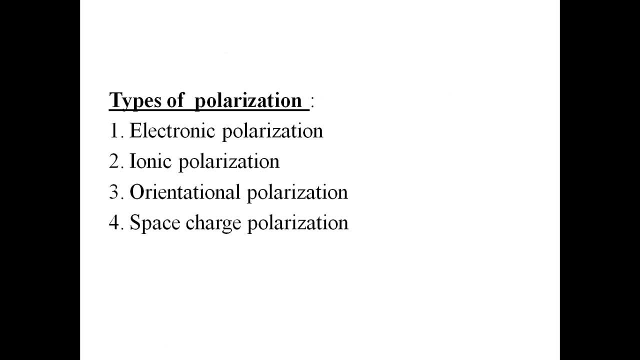 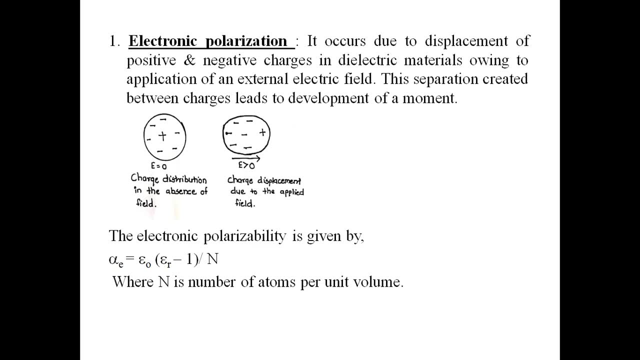 orientation, polarization, space, charge, polarize, polarization. now let us say one by one: first polarization mechanism is electronic polarization. you can see in this diagram, in that first diagram, there is a equal to zero, and there is he is applied. okay, now see, it occurs due to the displacement of 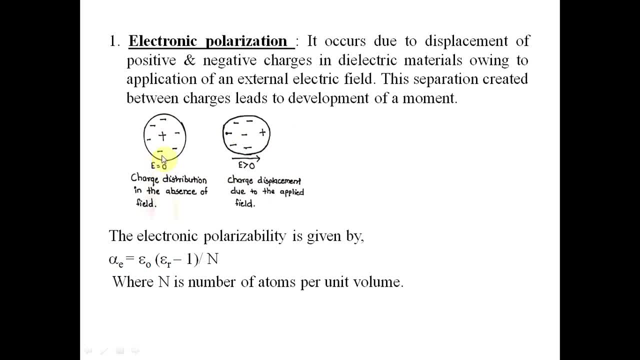 positive and the negative charge in the dielectric material due to the application of an external electric field, and this separation- is a created- between the charges leads to a development of their dipole movement after applying the electric field. so there is a dipole movement is a created. the electronic polarizability is given by alpha e equal to 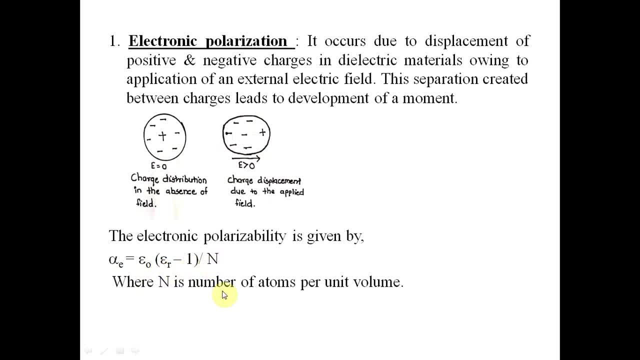 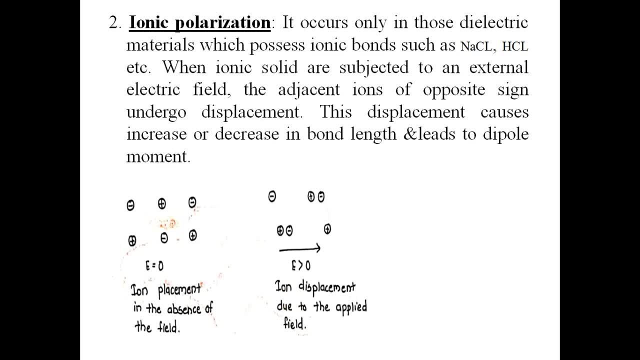 Epsilon 0 in back, Epsilon R minus 1 by n. very n is a number of atoms per unit volume. now the second one is ionic polarization. similarly here also see in this diagram: in first diagram e equal to 0, and after that electric field is applied, this dielectric ionic polarization occurs. 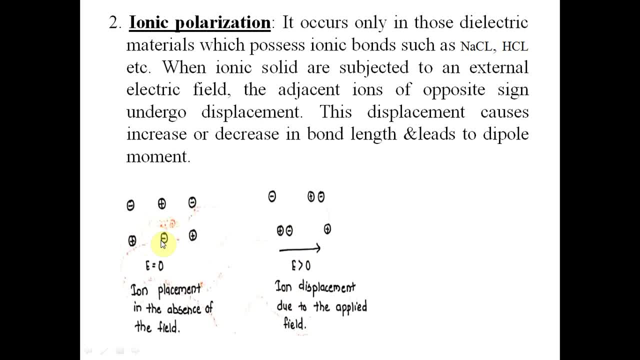 only in the ionic bonds such as a NaCl, HCl, etc. and when these ionic solids are subjected to an external electric field. see in this negative and the positive charges are there, it undergo the displacement. and how to take the displacement, the displacement, this takes place.